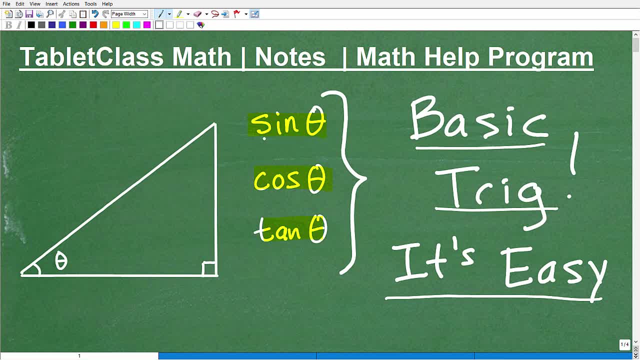 If you have one handy, you'll see these little functions we call them, and they have to do with trigonometry, And trigonometry is an awesome mathematics. okay, because it can solve all kinds of cool problems that involve angles and distance and whatnot. I'm going to get into all that in a second And, irrespective of where you're at in math, okay, even if you only know basic math, you'll understand this. Okay, you'll understand the essence of basic trigonometry, And the whole point of this video is to 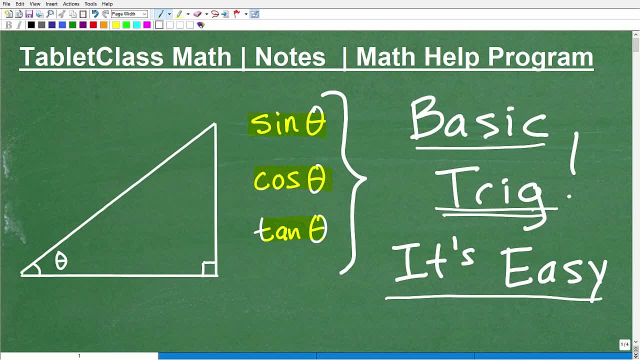 introduce you to trigonometry and hopefully get you excited enough to like actually want to learn more about it. But before we get into all that, let me go ahead and introduce myself. My name is John. I'm the founder of Tabit Class Math. I'm also a middle and high school math teacher And over many years I've constructed a ton of online math courses. I like to believe some of the most comprehensive math courses out there are all video based, full direct instruction, thousands of problems solved with video solutions. So you want to check out my 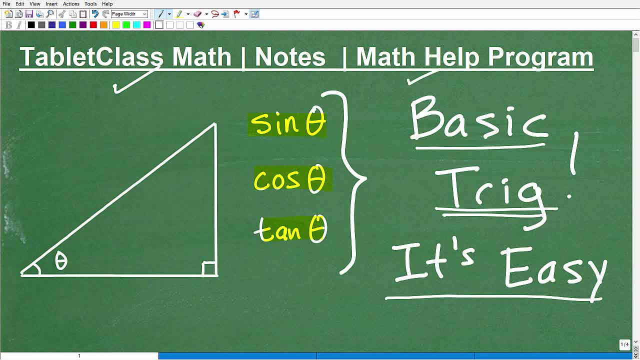 math program. I'm going to leave a link to that in the description of the video. So, whether you need to take a full online math course or you need help with the current course, that you're in, my program can help you Also. hopefully you're taking good notes. If you're not, you need to. Okay, the secret to doing well in mathematics- and this is over many, many years of teaching- is your notes. you got to like look at your notes and ask yourself: how strong are your notes? you need to take good notes And you need to study for. 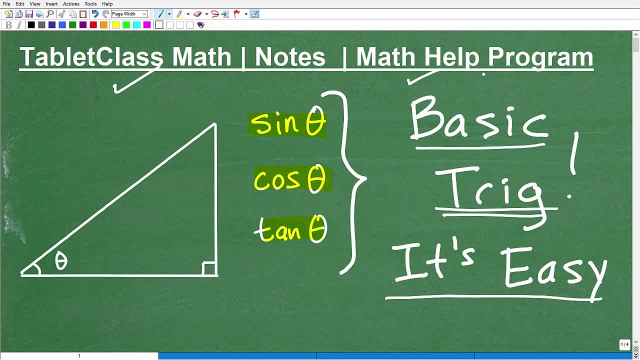 me notes. Okay, it's very, very important. So I've actually done several YouTube videos on note taking, the importance of that. you can find those on my channel. But if you, you know, have not been taking good notes and you need a good set of notes, which you do, I offer pre algebra, algebra one, geometry algebra, two, trigonometry notes. I'm gonna leave the link to those in the description of this video- super comprehensive, but I 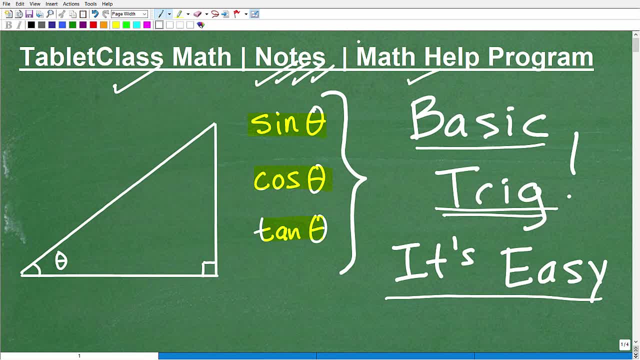 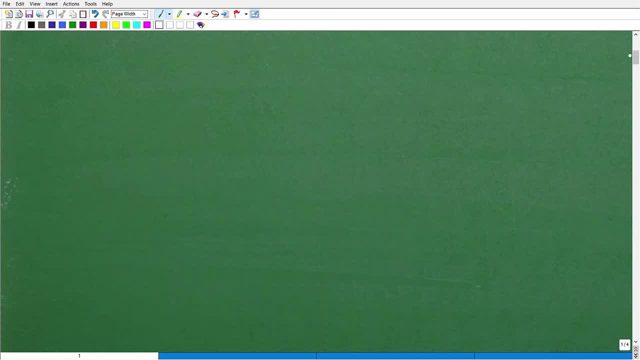 again, you've got to be able to take good notes yourself. All right enough said, let's get into trigonometry And let's take a look at some problems that trigonometry helps us solve. So let's say, here is the ground And here is, let's say, a tree, Here's a tree. Okay, And a tree obviously is pretty high. And what if I want to know the height of the tree? Okay, well, I got a couple choices right. I can try to. 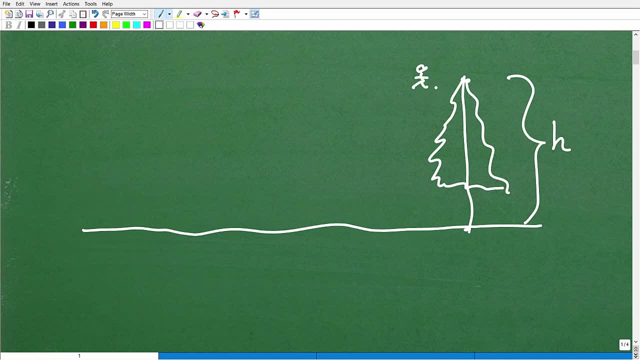 you know, like maybe climb a ladder kind of way up here and drop a tape measure down. Yeah, that's not really practical. What if this tree is, like you know, I don't know- 150 feet tall? you know those huge trees. Well, there's another choice we can do. We can walk way out here. let's walk out, let's say, 300 feet, And let's suppose we had a some sort of instrument that could tell us the angle from 300 feet And we just kind of like 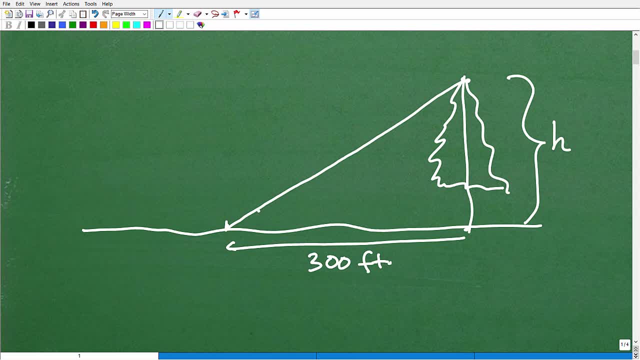 look up, All right, And it tells us this angle, right here, So from the ground, all the way up, okay, we kind of use this like little telescope type of deal. You look inside of it and it tells us the angle. But let's suppose that angle was, oh, I don't know, let's say, 30 degrees. Okay, So from 300 feet away from the base of the tree, we stop and then we look up and we measure this angle. Well, guess what? that's all the information we need. 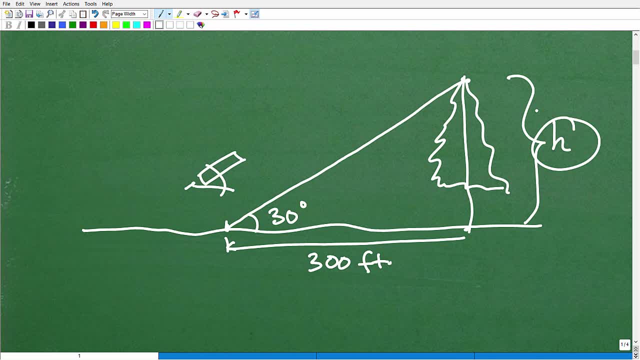 We need to determine the height of the tree. Okay, so you can see: wow, that's pretty cool, But we need trigonometry. Okay, we need trigonometry to do that. So trigonometry allows us to find the lengths of triangles. okay, whether it's this, this length, we could also find this length. Okay, If we only have an angle and one length of the triangle. Okay, So this is really really. 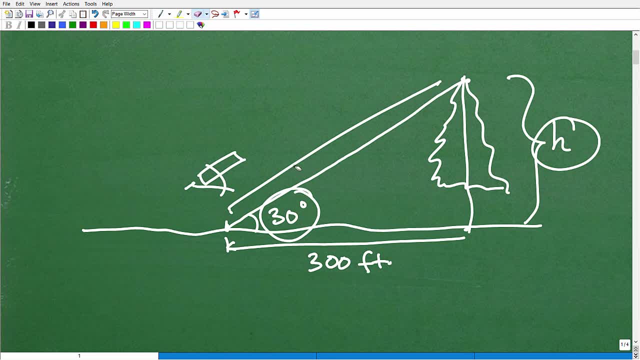 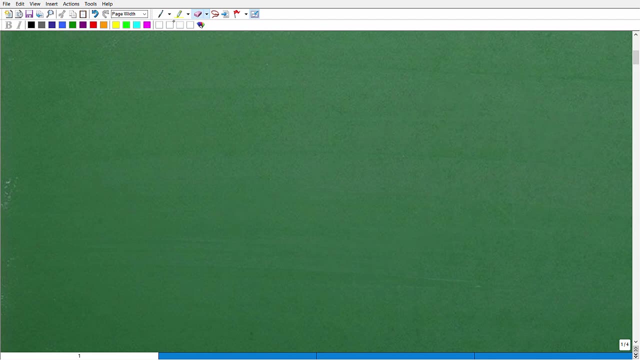 powerful stuff And you know you can think of all kinds of different examples. you know, like word problems that trigonometry helps us solve. Okay, Now let's take a look at a basic triangle problem And then we'll get into this trigonometry stuff. So here let's say I have what we call a right triangle, Okay, And let's say this is three and this is. 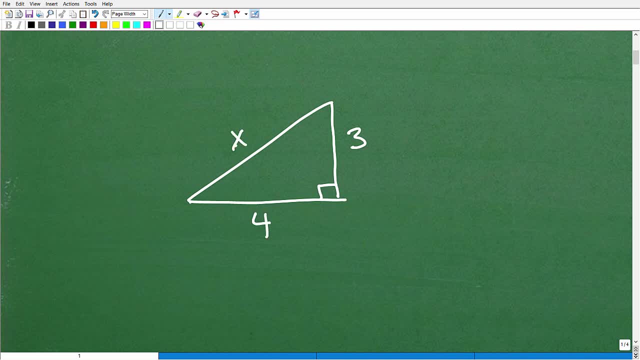 four And this is five, And this is six, And this is seven, And this is eight And this is four, And I wanted to know this length right here. Okay, Well, with right triangles, right, these type of triangles, this right here is a 90 degree angle. I can use this guy: a squared plus b squared is equal to c squared. Okay, this is called the Pythagorean theorem, super, super, super important in mathematics, okay, and in trigonometry as well. But this theorem or formula, okay, however you want to think of it. 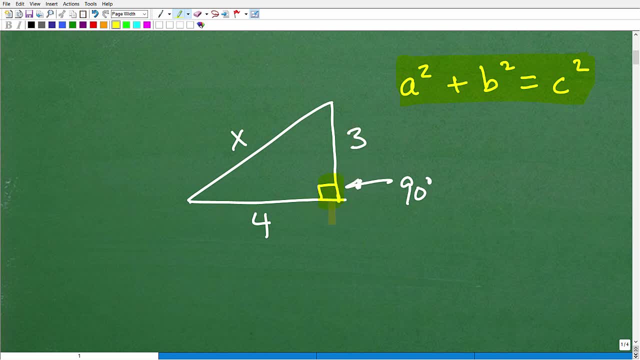 will allow us to find the lengths of a right triangle. Okay, so if I got two lengths, I can find this length. all right, I can just plug everything in. this would be three squared. this would be our a, this would be our b. Okay, so, real quick, this is what. let me erase this. this is nine plus 16 is equal to c squared. or 25 is equal to c squared. take the square to both sides: c is equal to five. Okay, So the length of this is equal to 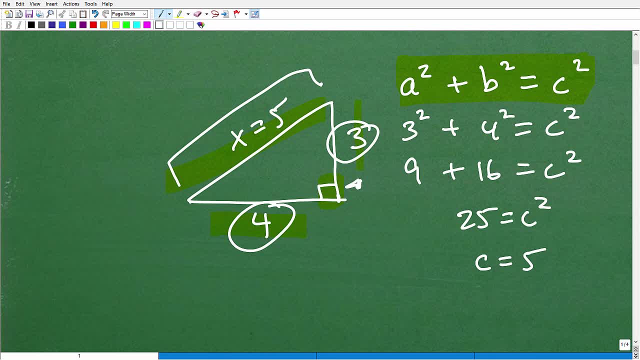 five. But here's the deal. Sometimes, you know, in practical measure I'm not going to have the lengths of two sides, sometimes just like my little tree problem here. Okay, let's erase all this. All I'm going to have is my little tree, All right, And I'm going to have maybe one length, Okay, But if I can get an angle, all right. then I could determine, I'd like to be able to determine all this information, All right, But this theorem. 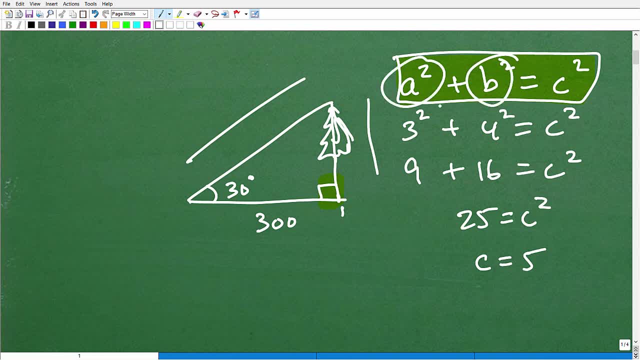 is going to require us to have two pieces of the of the puzzle to get the third. trigonometry says: Hey, if you just give me an angle and you give me one piece information involving a right triangle, I can get you anything you want. I can get you this angle, I can get you this distance, this distance, etc. So basic trigonometry is revolves around these basic right triangle problems And, of course, trigonometry is a huge topic. 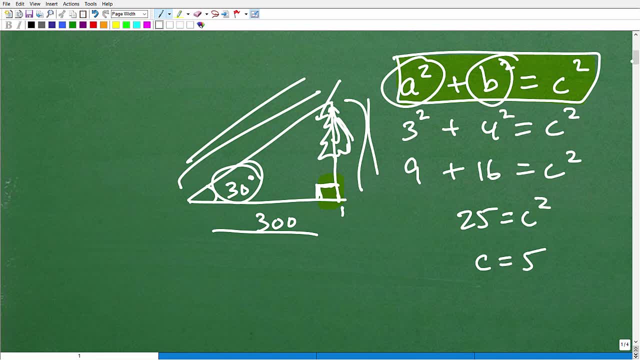 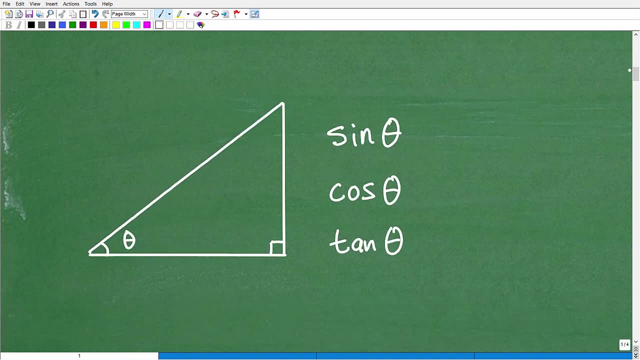 And it gets into much more sophisticated concepts. But again, this video is about basic trigonometry, So let's get to it real quick here Now, now that you know why we need trigonometry, why it's important, And let's talk about these functions here. These are the basic functions of trigonometry And we're going to teach them to you now. All right, so let's take a look. This is a right triangle, Okay, and this right here would be an angle in that right triangle. right Now, if you don't know this, I'm going to 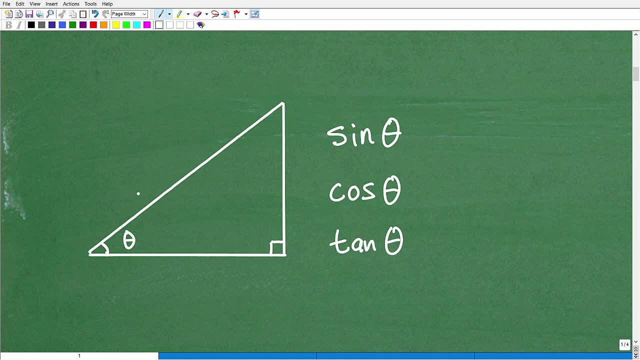 tell you this: Now, in a triangle, a right triangle, the longest side is always this side. It's called the hypotenuse. Okay, Now this angle here, if I look way to the other side of it, okay, I'm going to call this the opposite side. Okay, the opposite side, All right. and then this side: okay, with respect to this angle, I'm going to call the adjacent side. So this length right here we'll call the adjacent to this angle because it's next to it, right? It's kind of like touching the angle And then the 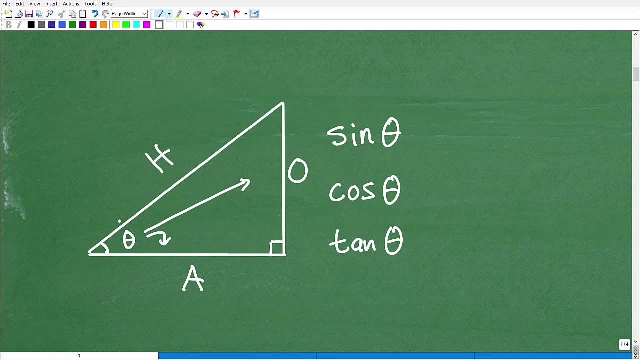 side that's opposite. we'll call it the opposite. Oh, okay, And then this side right here is the hypotenuse. Okay, let's see how that works. All right, so H, O and A represent the lengths of this particular right triangle. Now, excuse me, let's talk about these functions here, Sine. 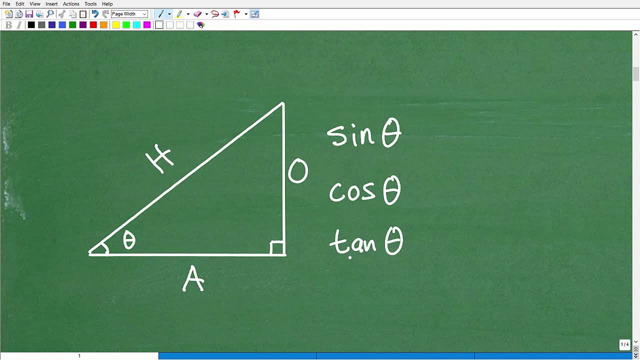 cosine, and that's how you say this. This is called the sine, This is called the cosine, This is called the tangent. All right, so now I'm going to give you a phrase. So katoa, Now I know you're really like: what is this guy talking about? Well, 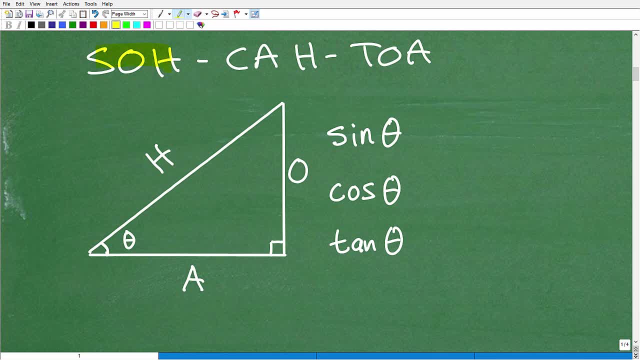 it's going to make sense here in a second. All right, so the sine, the sine of an angle, okay, the sine of this angle is what we call. we think of so. Okay, so you're like. so, all right, O and H: Okay, it's going to be the sine. 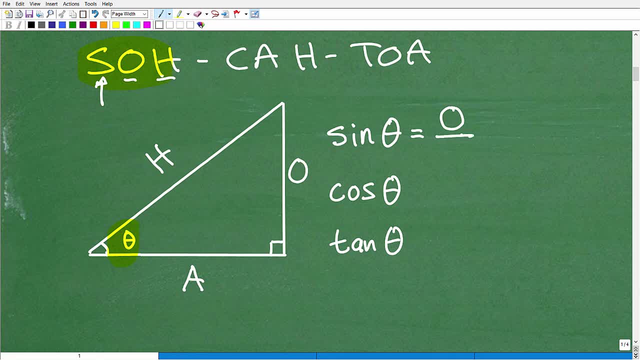 is the opposite, the opposite over the hypotenuse. Okay, so what's the opposite? Well, here's the O. Okay, right here. So, whatever this length would be. okay, I take this length and divide it by this length. All right, that's it. Okay, now so the sine of this particular angle. 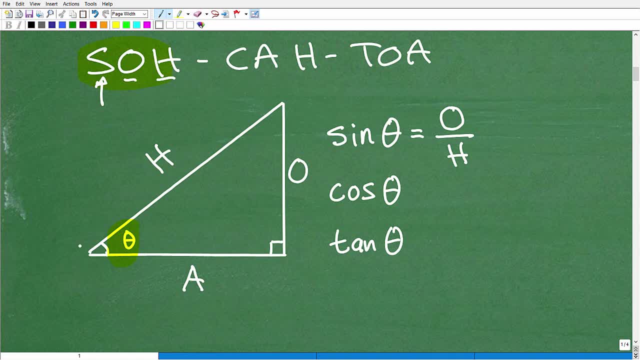 is going to be. whatever this length is divided by this length, That's it. Okay, how about cosine? All right, so cosine is the adjacent over the hypotenuse. So that's going to be. let's give ourselves more room. 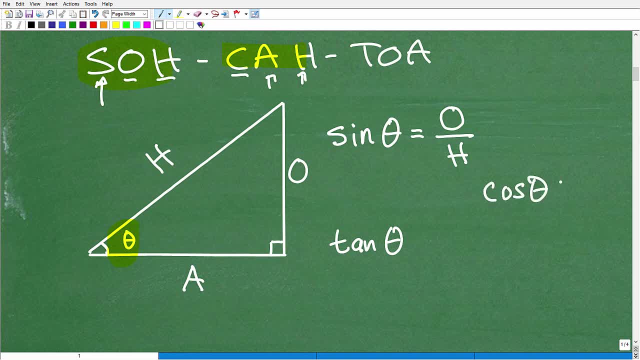 Let's put cosine over here. Cosine, that little thing is called theta, is the adjacent over the hypotenuse, And then tangent. here this is called, the tangent is going to be- you guessed it, the opposite over the adjacent. So O over A, And these are just ratios of this right triangle. 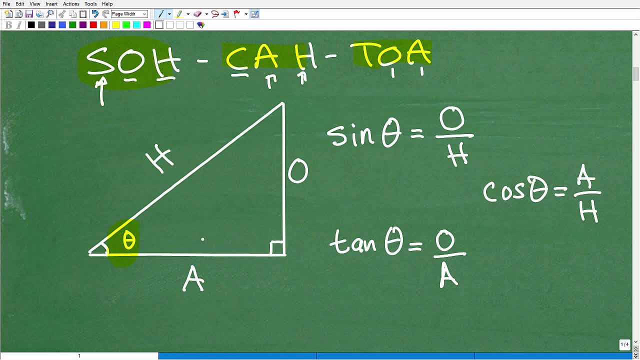 These are the lengths. Okay, so, if you remember, we had that previous triangle. this length was four, this length was three and this length was five. Okay, so the sine of this triangle here would be what? Okay, well, our O would be three. right, that's the opposite length divided by the hypotenuse. 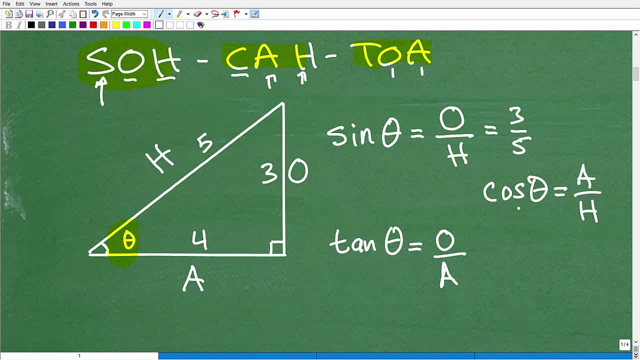 which is five. So the sine of this particular angle is three-fifths. Okay, the cosine would be four-fifths. Tangent would be the opposite over the adjacent three-fourths. Okay, so let's take the tangent. all right, The tangent was equal to three-fourths right. Three divided by four. the opposite over. 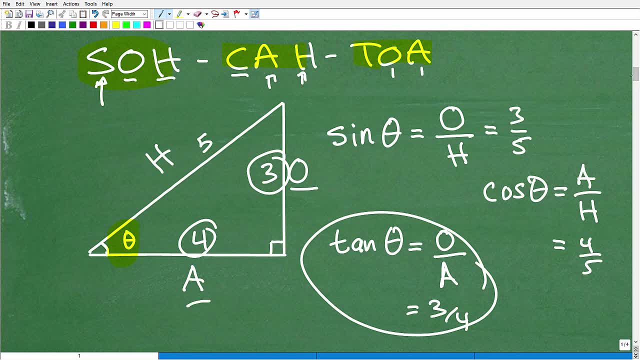 the adjacent. So how is this going to help us? All? right, let's say I have this triangle and it's three, four and five and I wanted to know this angle. Well, that little Pythagorean theorem that's not helping us out. Okay, we can't solve that, So what we would? 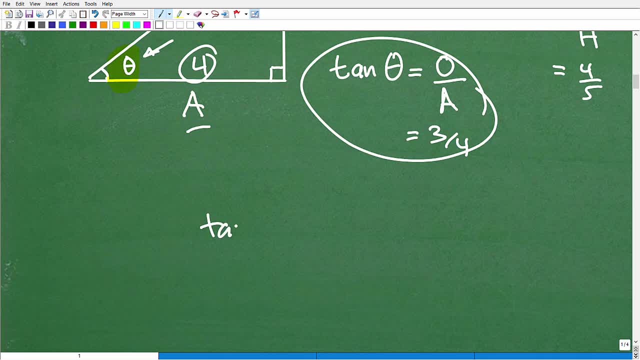 do okay. we'd say: well, the tangent of that angle is equal to three over four, or what's that? 0.75, right? So the tangent, the tangent of a particular angle, is equal to 0.75.. What is the? 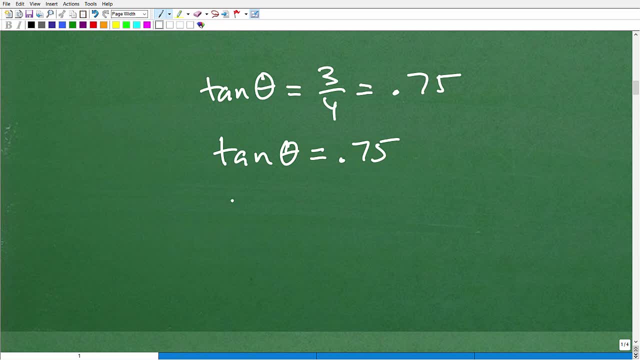 angle. Well, there's a function on our calculator and you do need a calculator or a table of values. It's called the arc tangent. okay, It goes, it looks like that, but all but this. what you do is just this is just using your calculator. I could find. 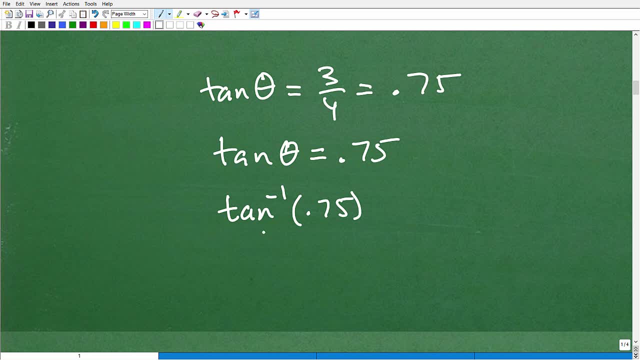 the arc tangent of 0.75.. Basically, I'm going to ask my calculator what angle has a tangent of 0.75, and it would spit out the number. okay, in a, in a, in an angle, right, I don't want to get. 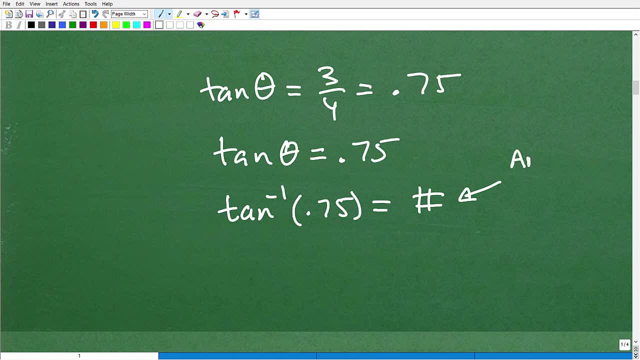 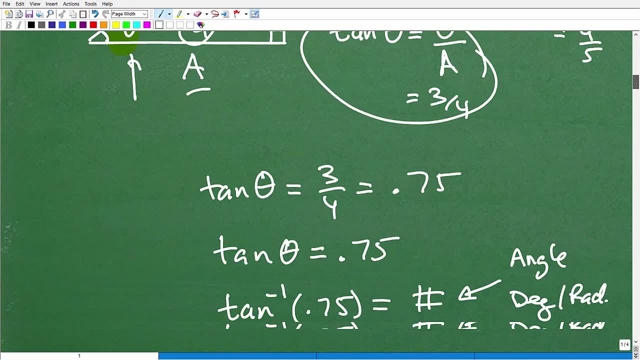 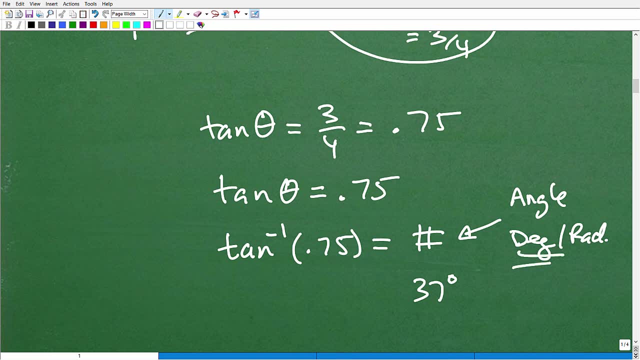 I don't want to actually have my calculator with me in front of me. Should have done it. but let's say it came out and popped out to be 37 degrees, whatever, it is okay. It will tell you that if, if your calculator is in degree mode, okay. And so with this is just only one example. 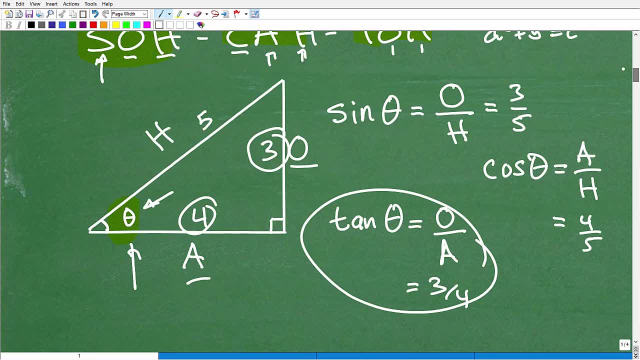 of what you can do in terms of solving right triangle problems. We can get degrees, we can get all kinds of stuff, and I don't want to make this video too much more in-depth, but just know, you've got your calculator and you understand these basic. 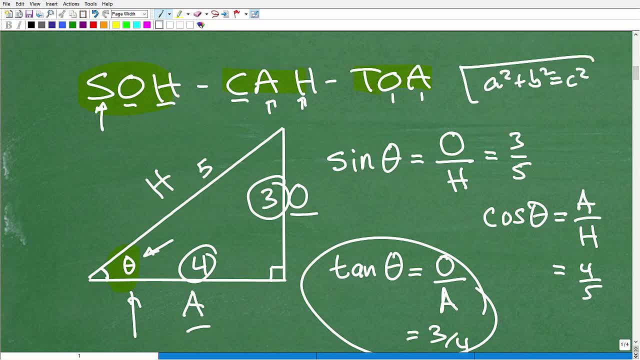 trigonometric ratios, trigonometric ratios, functions, and also it's handy to know the Pythagorean theorem. You can solve any kind of problem, like that little problem with the tree that we talked about, and much more. you know sophisticated type of problems. okay, So this is 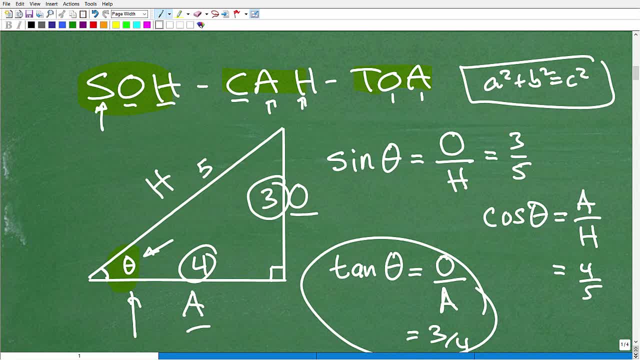 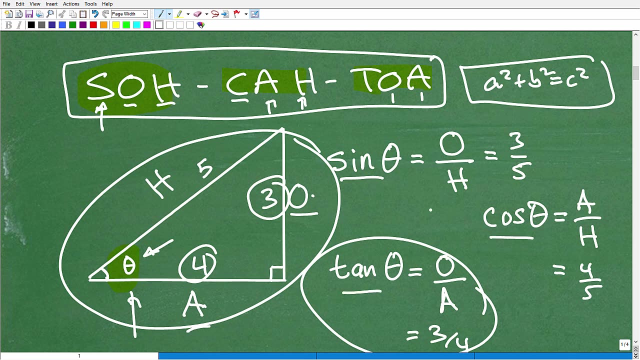 basic trigonometry, It's no more than that and really you know, if you know this, so katoa, and you understand this basic right triangle that we discussed, the opposite, the adjacent, the hypotenuse and the sine, cosine and tangent, the ratios of these various sides and how we can use our